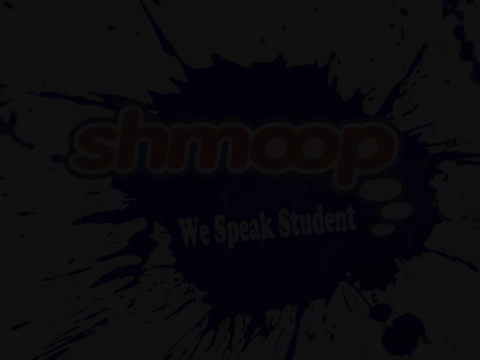 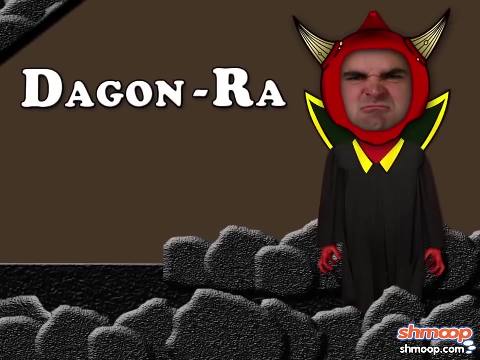 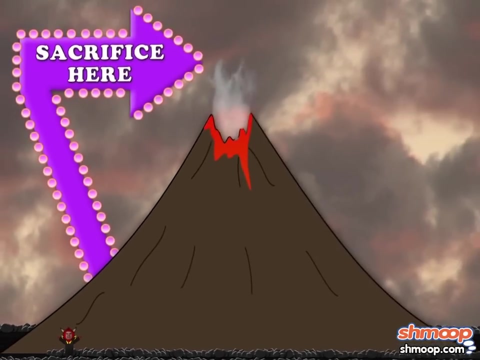 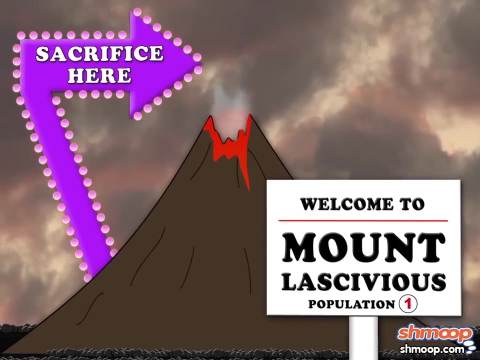 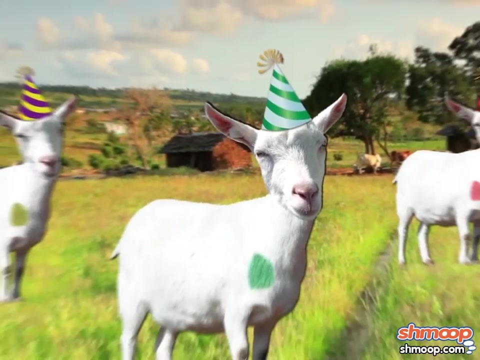 Counting Principle a la Shmoop. Dagon Ra Lord, High Chancellor of the Volcano People, is in a pickle. It is Dagon Ra's duty to choose those who will be sacrificed to Mount Lascivious, But he's so bad at making decisions. 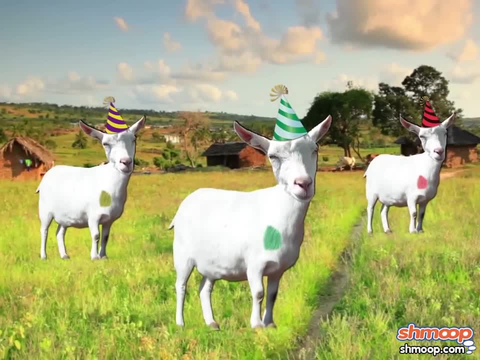 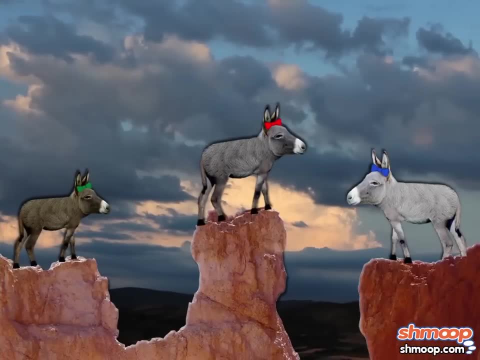 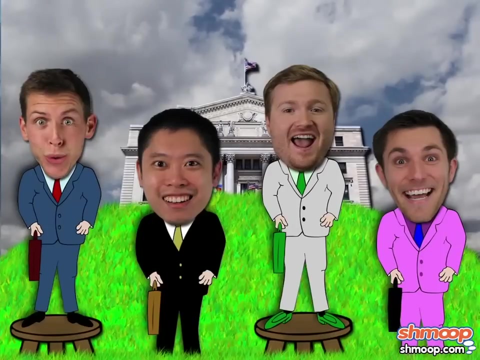 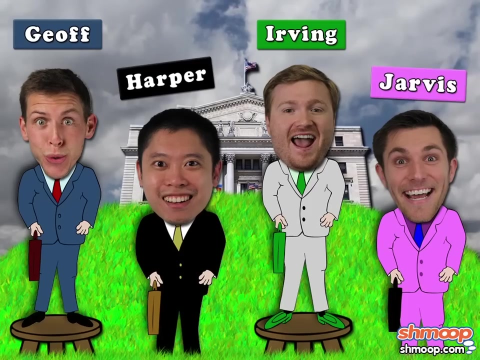 He must choose to sacrifice one of the town's goats, Alfred Bobo or Chewy, One of the town's donkeys, Darius Eeyore or Fartsy, And one of the town's lawyers, Jeff Harper, Irving or Jarvis. 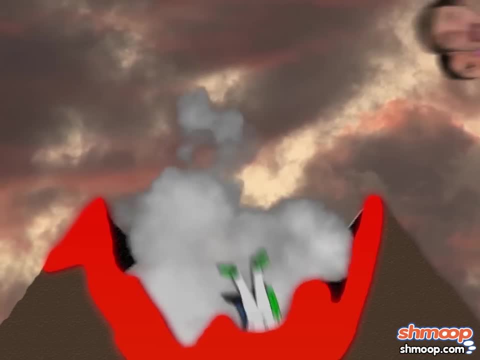 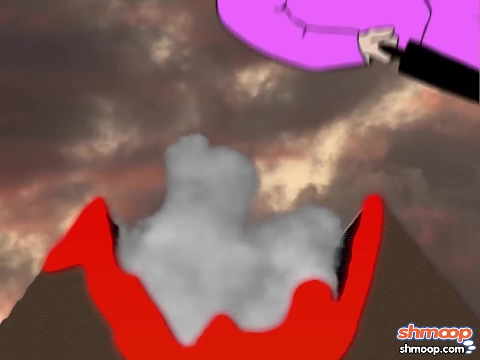 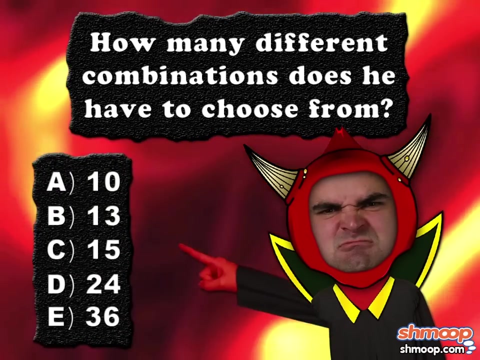 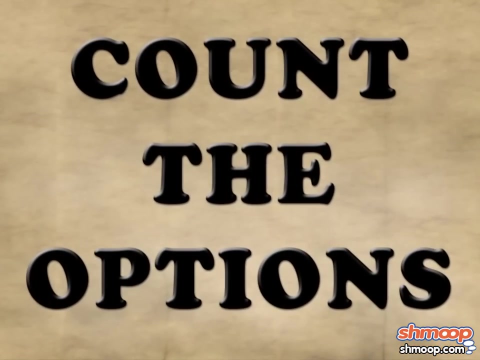 He briefly considers just tossing in all of the lawyers, but he doesn't want to upset the volcano. god, How many different combinations does Dagon Ra have to choose from? Here are your options. First things first. We need to count the number of options for each category. 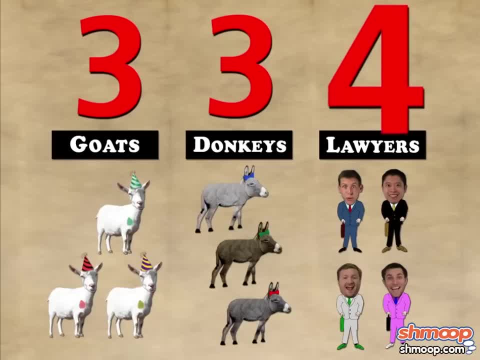 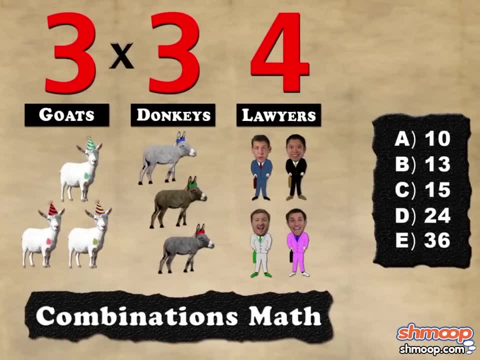 Looks like we're working with three goats, three donkeys and four lawyers. To find the total number of combinations, we would simply multiply those three numbers together. Three times three times four equals thirty-six. Answer E: Still confused. 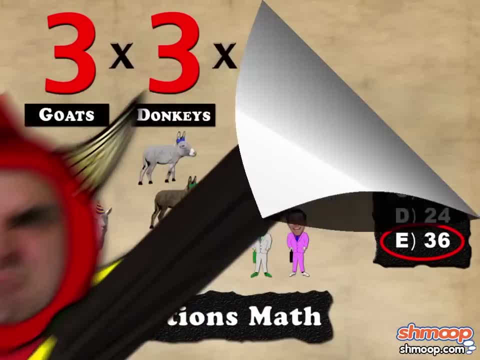 Here's what we really did. Let's look at all of his options. If he starts with the letter E, he's going to have to count all of his options. If he starts with the letter B, he's going to have to count all of his options. 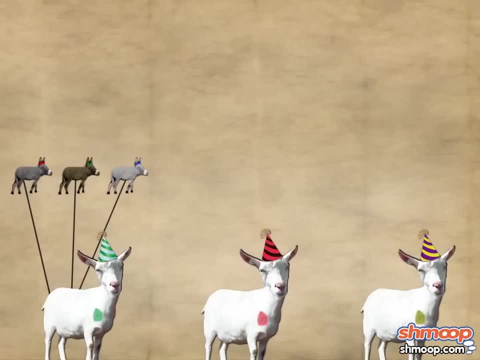 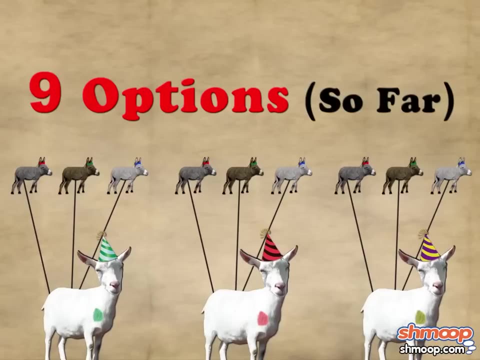 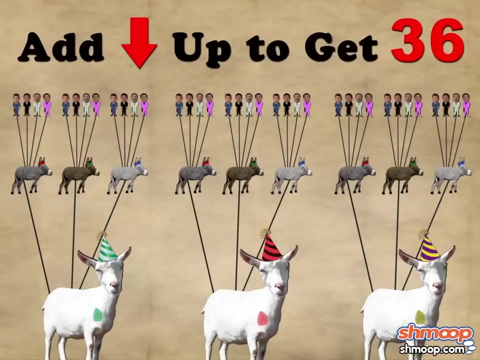 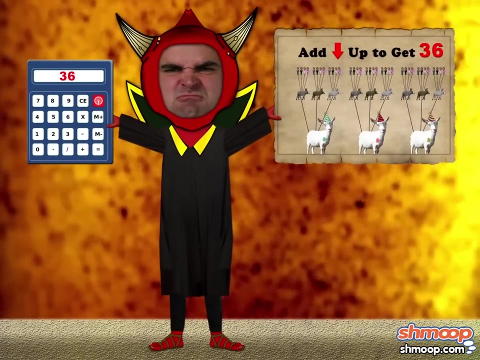 I could just make the whole thing surplus for him to just three goats. And if he starts with the letter P he would just have to keep counting all of his options. So that gives him three options. To get back to him, I'm gonna need to use my